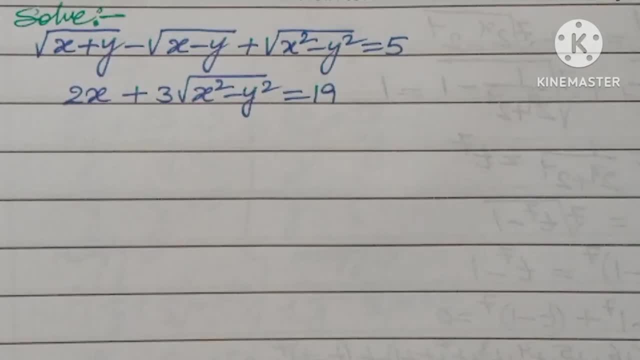 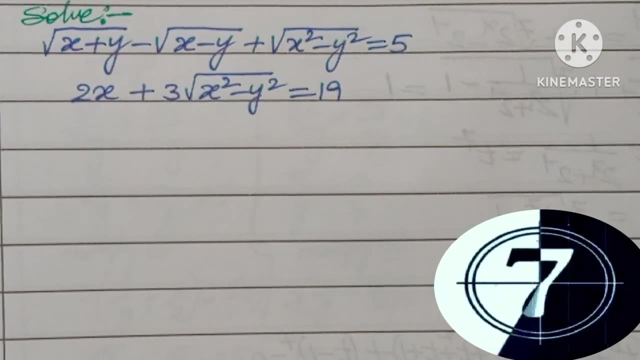 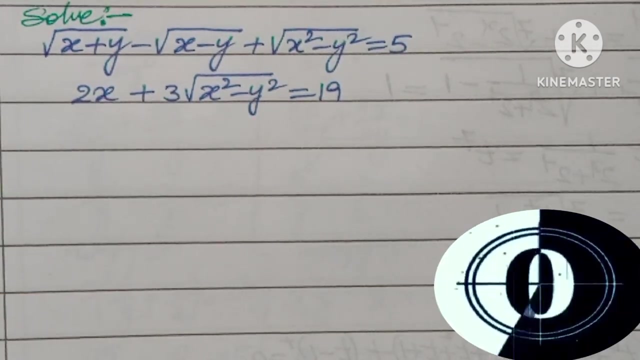 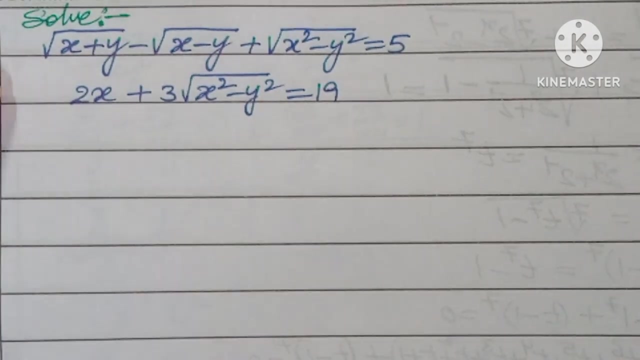 So, as you are going to solve this logical, critical and olympiad problem, pause the video for 10 seconds and try it out. Okay, and also, if you are new to the channel, please subscribe the channel and give it a thumbs up. It will appreciate us to make more videos, more than thousand olympiad. 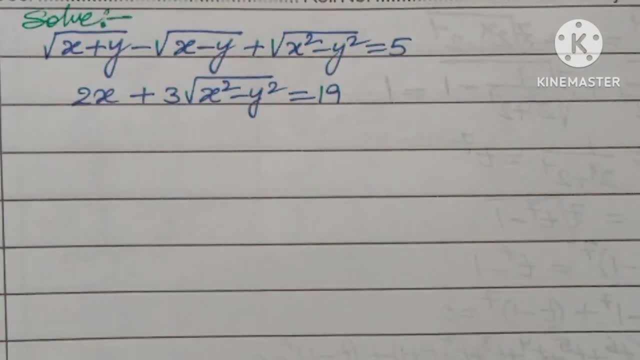 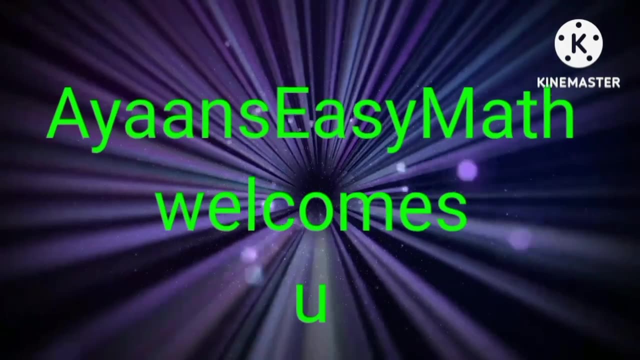 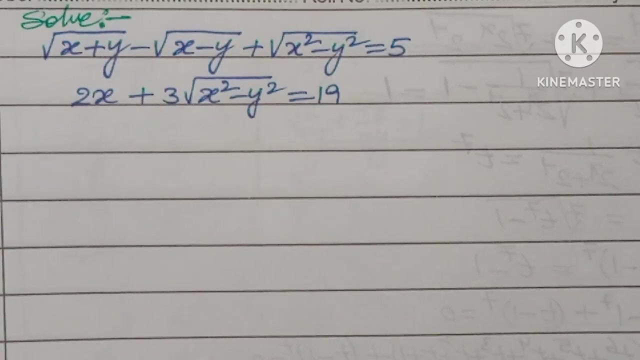 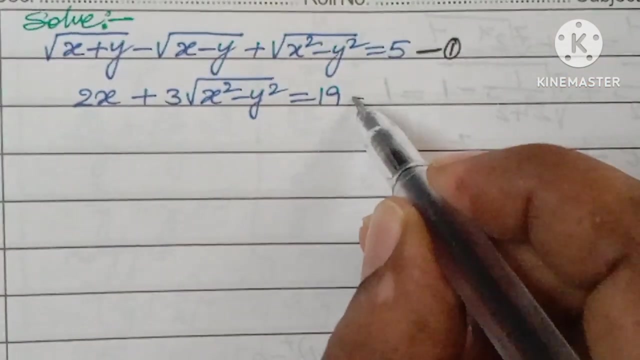 and logical problems. If you have any questions or uploaded in this channel, please go through them. Thank you, So how to solve this problem? Let us take this as equation 1 and let us take this as equation 2.. So I am going to do some adjustment in. 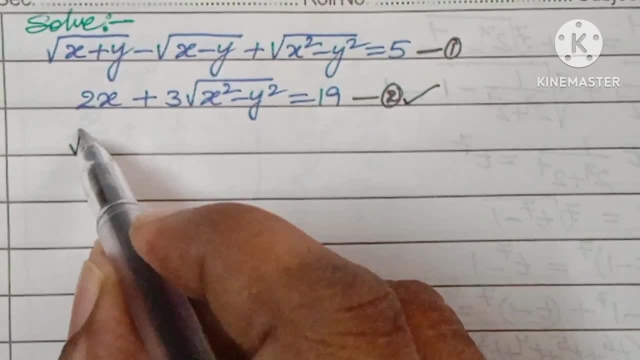 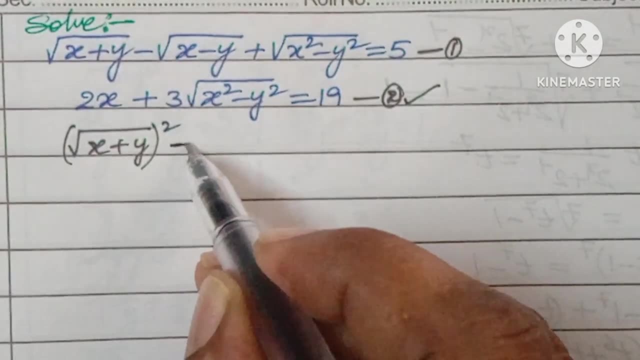 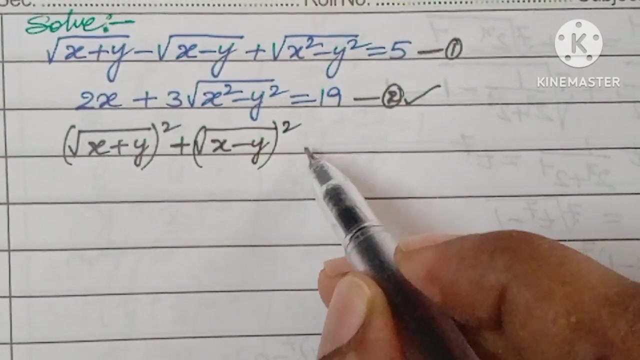 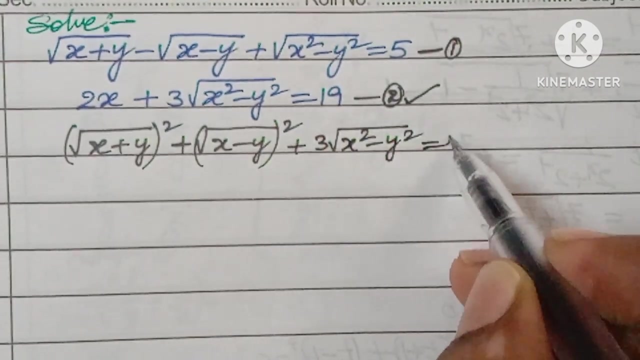 equation 1.. So here, 2x I am writing as: root of x plus y, whole square plus root of x minus y whole square plus 3. root of x square minus y square is equal to 90.. If any easy methods are there, you can comment in the comment box. 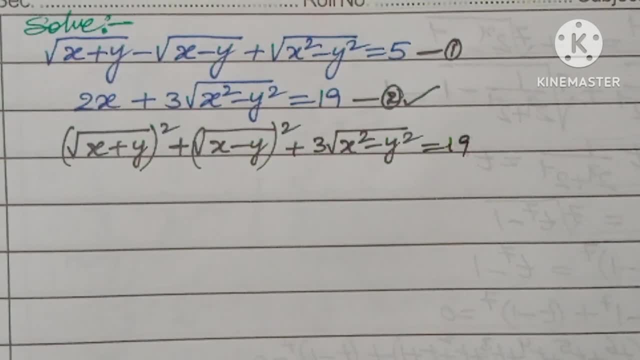 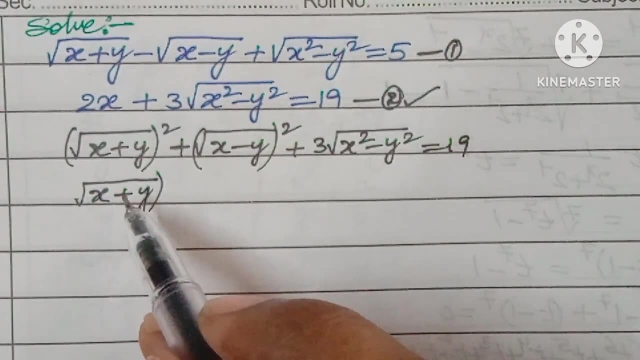 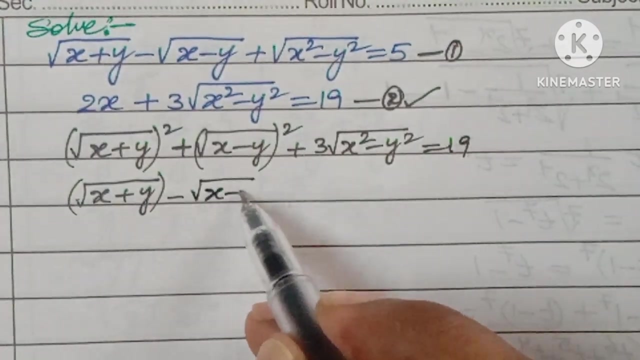 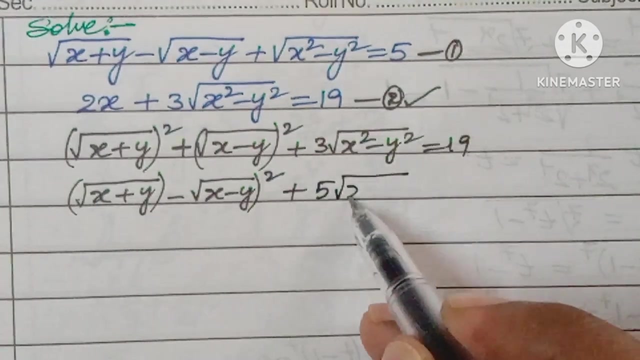 You can give the suggestions So this can written as root of x plus y whole square, or you can write it as root of x plus y minus. root of x minus y whole square plus 5. root of x square minus y square is equal to 19.. 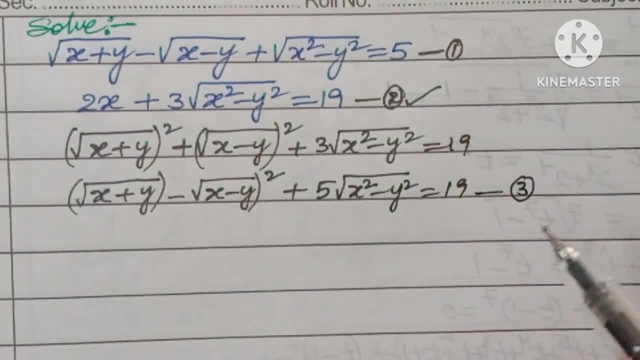 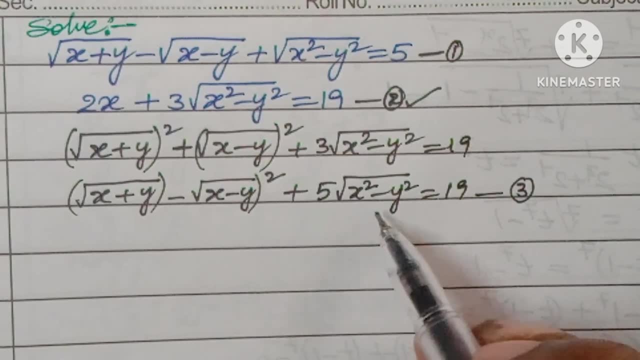 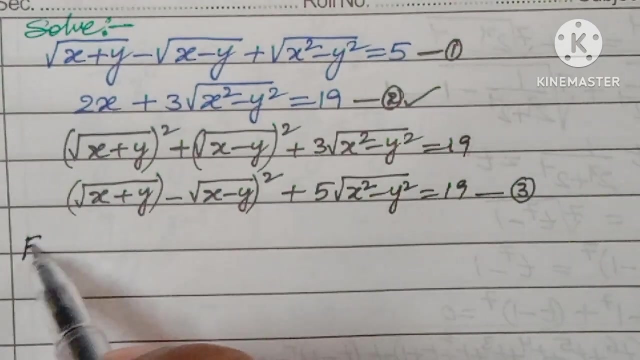 Let it be 3.. So here you will get minus 2 root of x square y square plus. you have to add both side, Emma. Both get cancelled. Now from 1 we are having root of x plus y minus, root of x minus y. 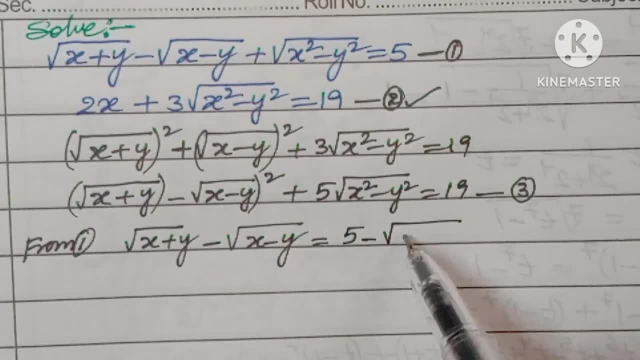 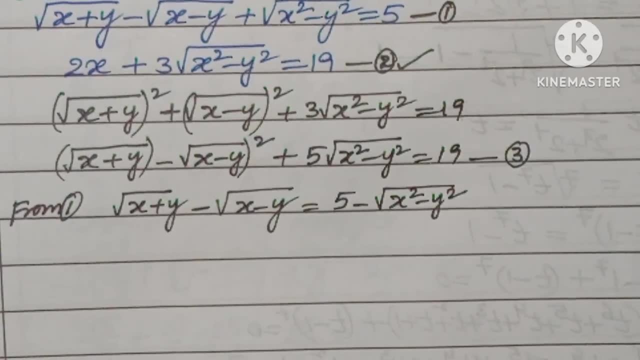 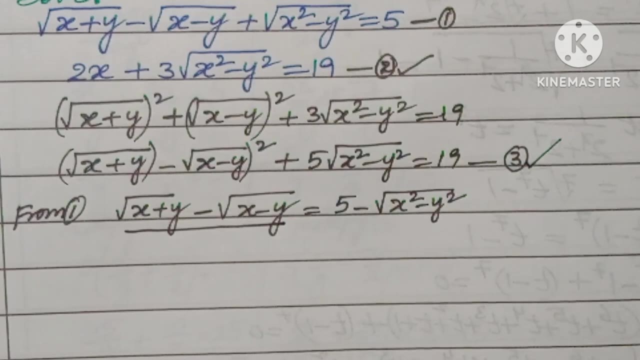 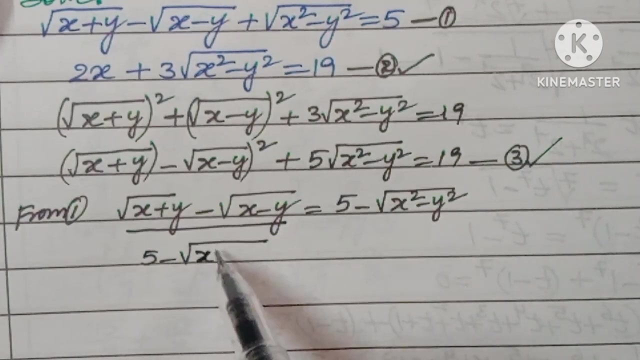 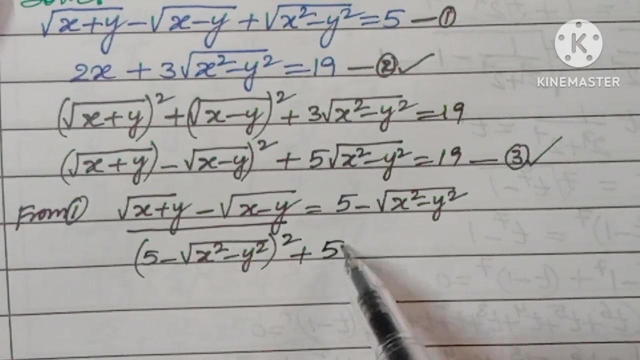 is equal to 5 minus root of x square minus y square. from first equation you are getting this. now replace this value in 3, replace this value in 3, then what will get? a 5 minus root of x square minus y square, whole square plus 5 root of x square minus y square is equal to 19. 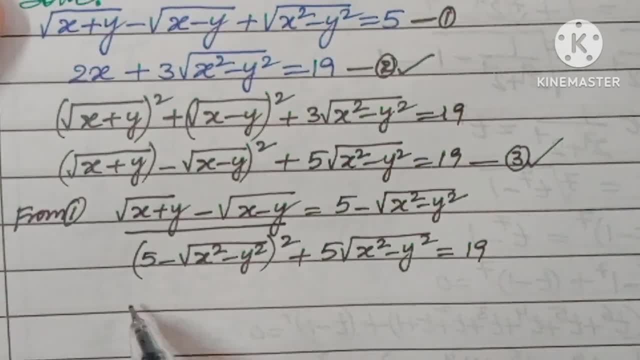 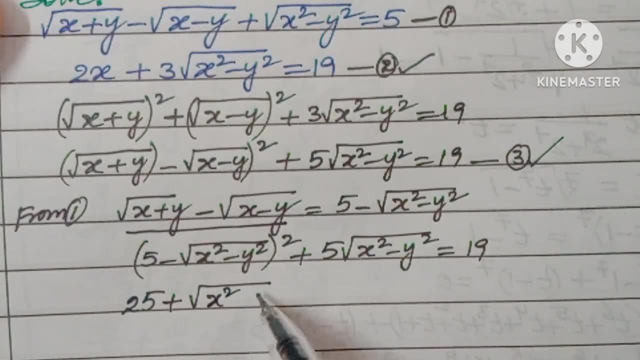 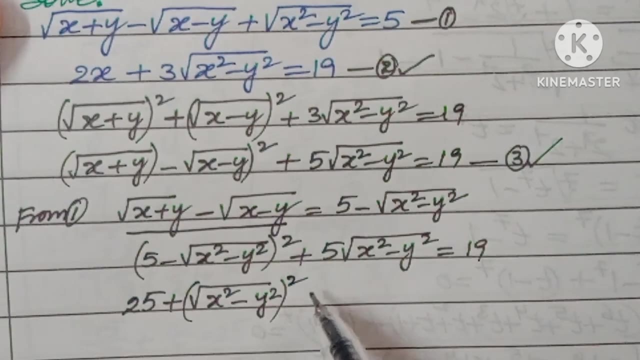 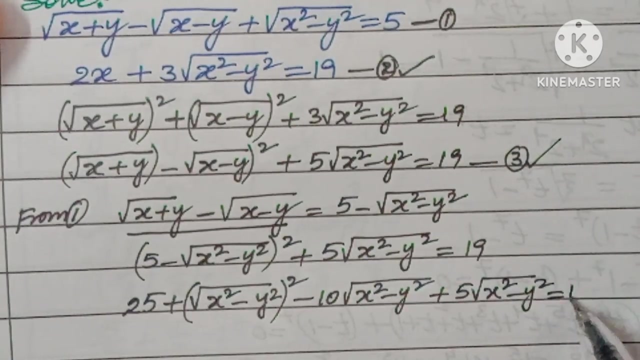 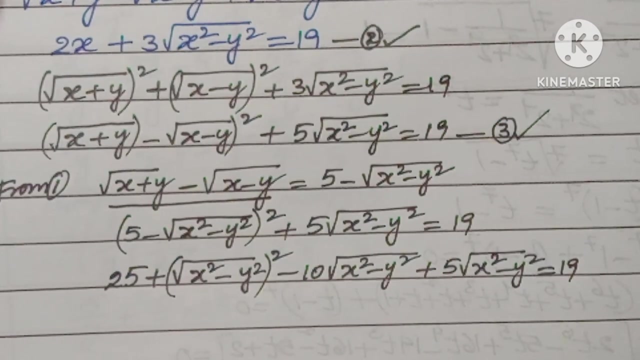 now, if you open this bracket, 5 square 25 plus root of x square minus y square, whole square minus 10, root of x square minus y square plus 5 root of x square minus y square is equal to 19. away now here, if you solve. 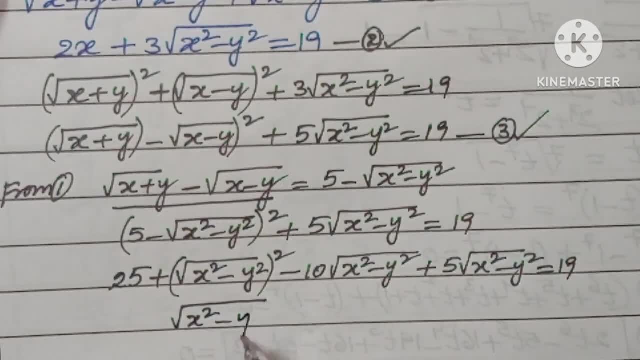 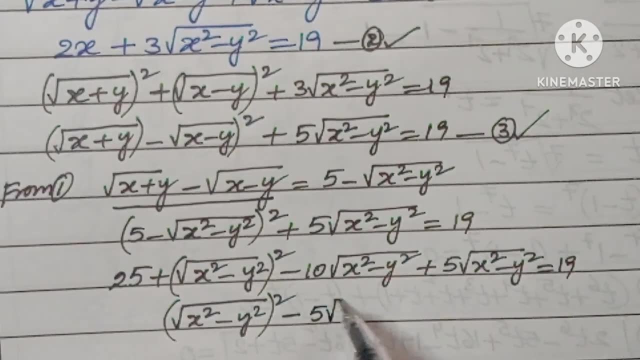 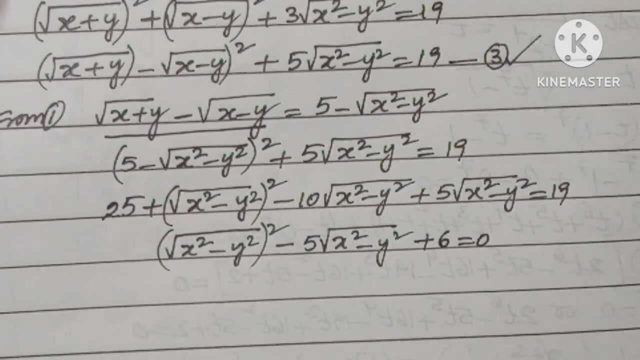 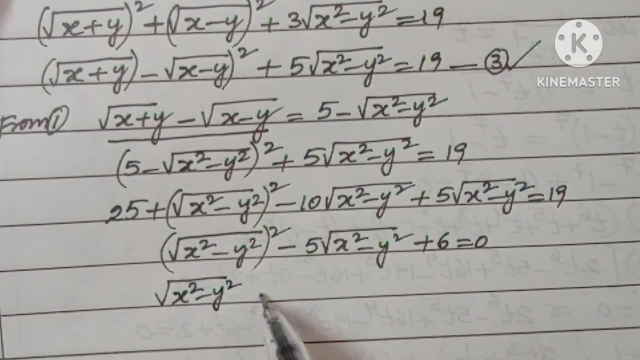 square and minus y square. whole square minus phi. root of x square minus y square plus 6 is equal to 0.. You got a quadratic in root of x minus y square. So root of x square minus y square you are taking as k. 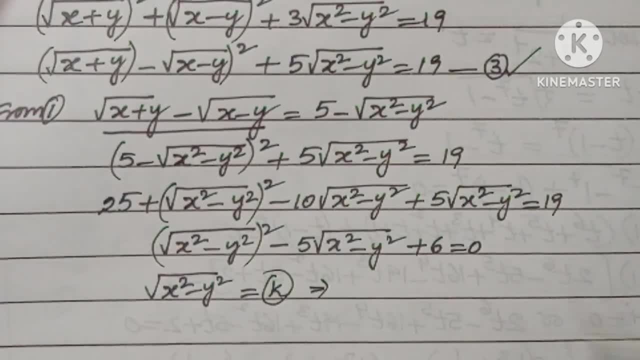 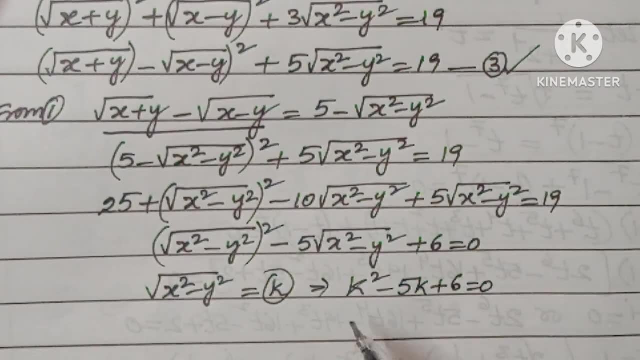 That implies what you will get here: k square minus phi, k plus 6 is equal to 0.. Now here you will get the factors k minus 3 into: k minus 2 is equal to 0.. Now here you will get two cases. 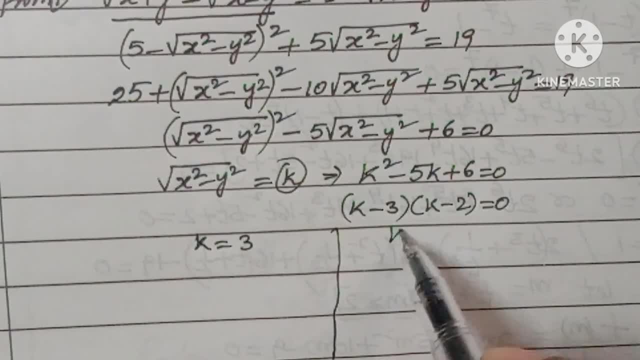 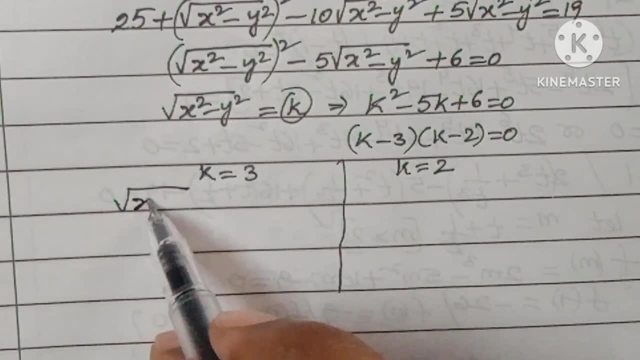 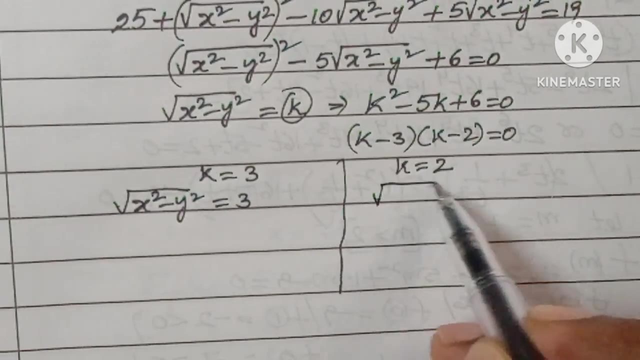 k is equal to 3 and the second case, k is equal to 2.. So what is the k value root of x square minus y square, equal to 3.. So here, what is the k value root of x square minus y square is equal to 2.. 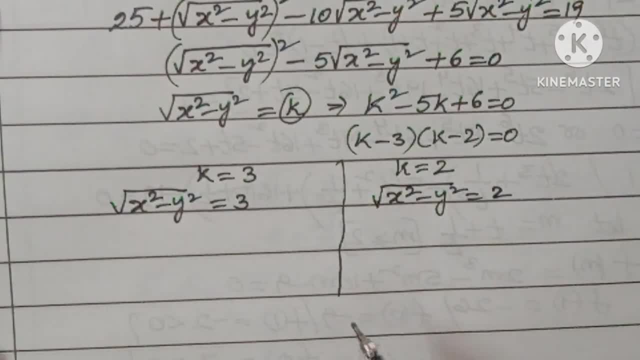 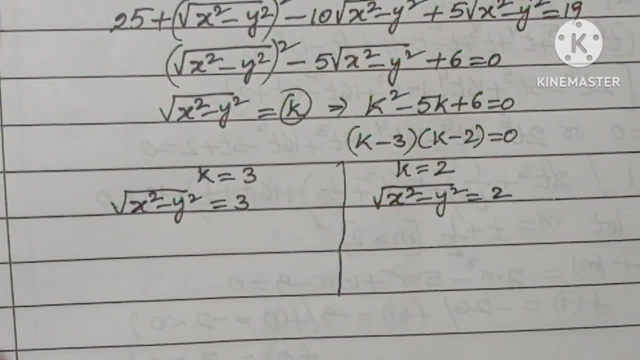 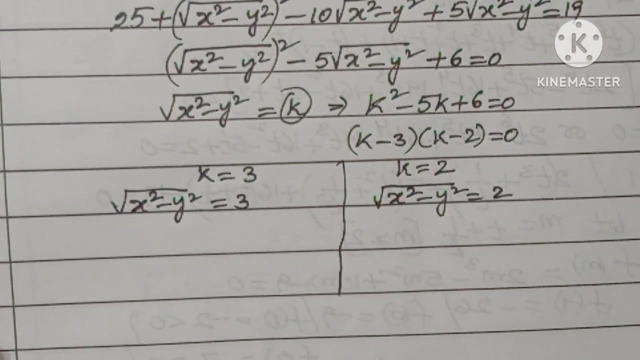 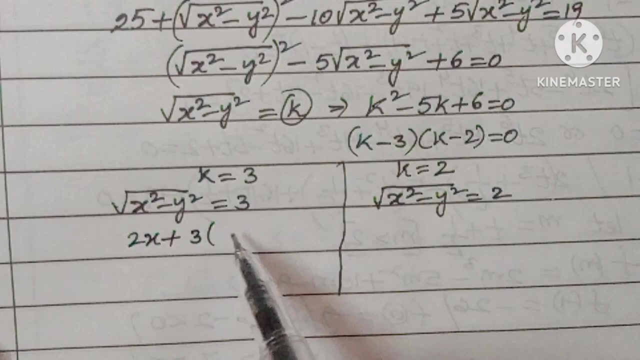 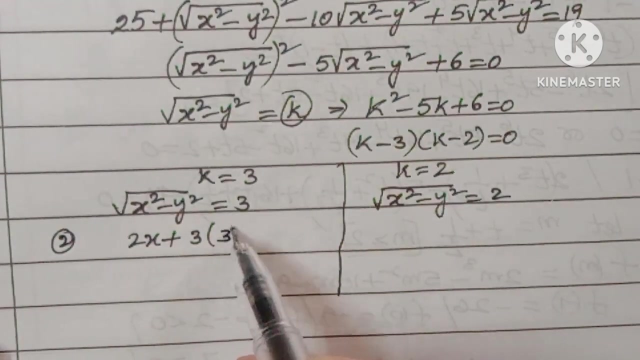 Okay, Now here Squaring on both sides, Okay, Here I will substitute In second equation. So here in second equation, if you substitute the value of k 2x plus 3 into Writing, k value Second one, So k value 3 is equal to 19.. 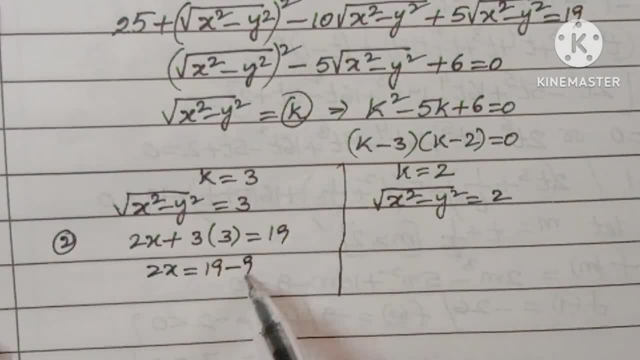 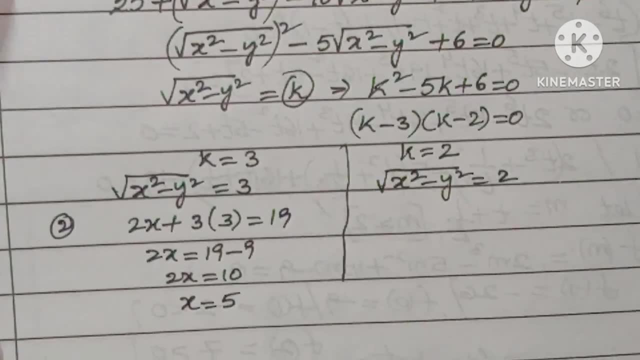 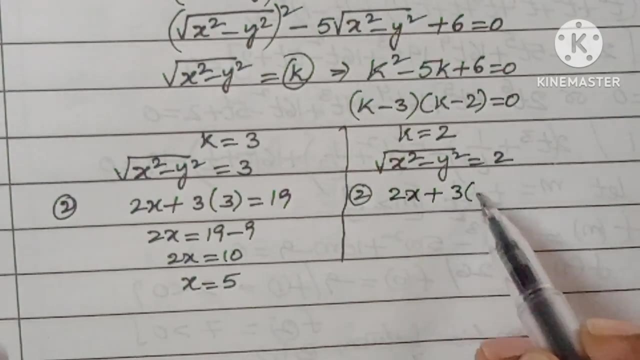 So 2x is equal to 19 minus 9.. 2x equal to 10, x is equal to 5.. Now if you substitute the value of k in second equation, 2x plus 3 into 2 is equal to 19.. 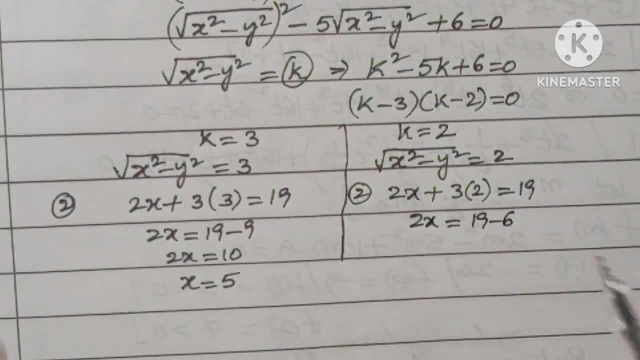 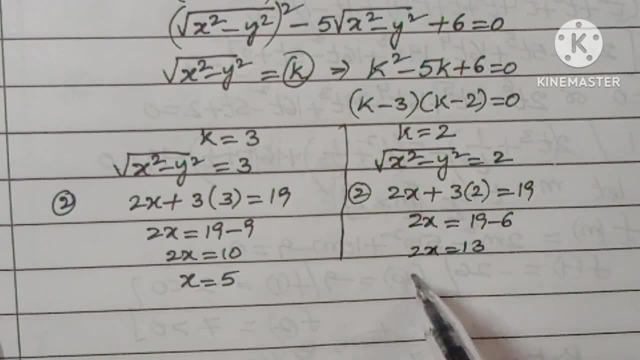 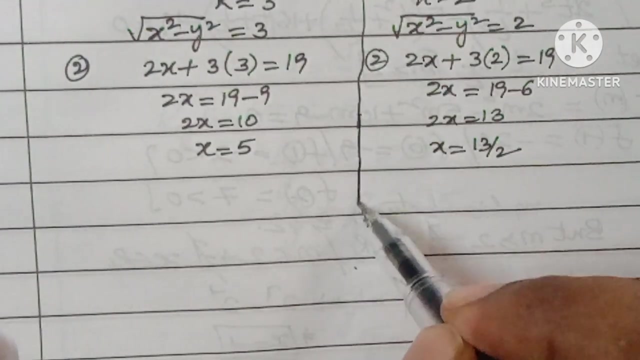 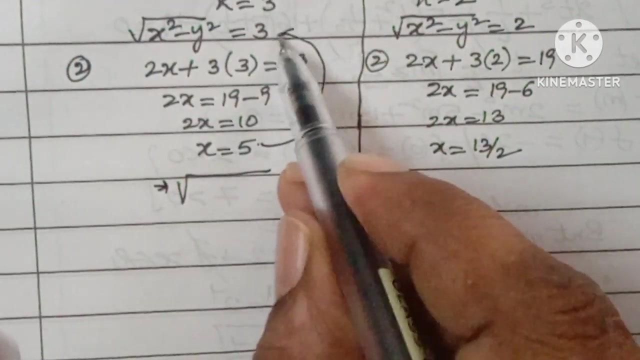 2x is equal to 19 minus 6, so 2x is equal to 30. now x is equal to 13 by 2. now if you replace this in k value. so what will get root of replacing this value here in this replacing this value here? 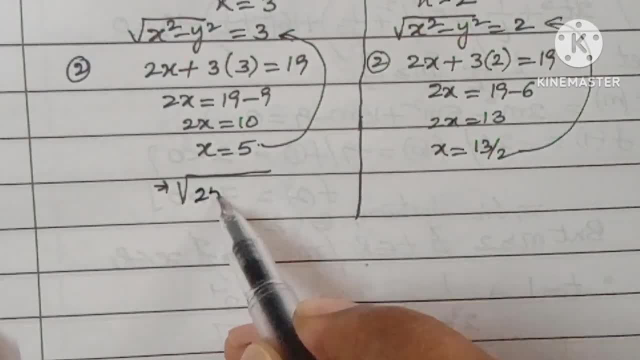 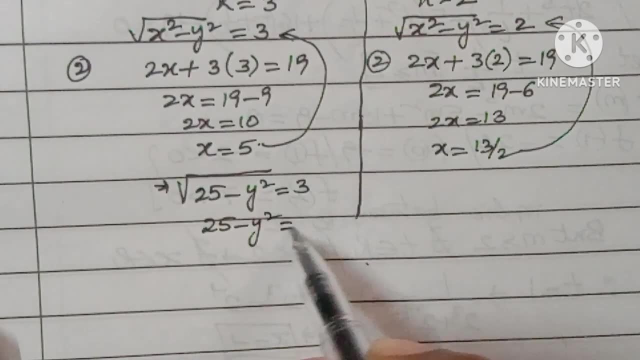 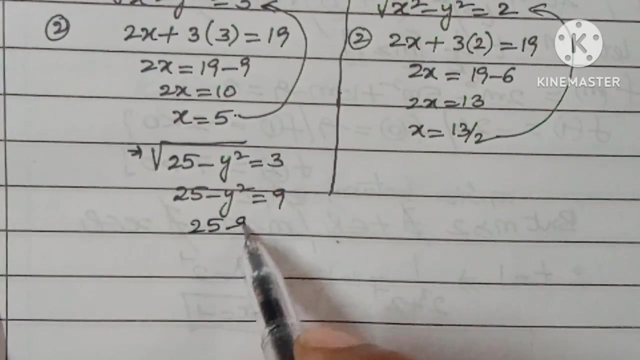 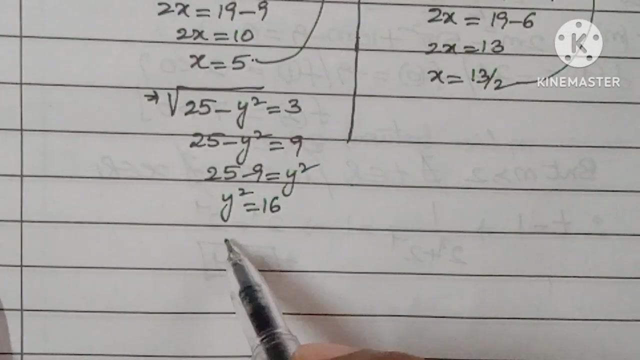 root of 25 minus y square is equal to 3. 25 minus y square is equal to 9, squaring on both sides. so y square, 25 minus 9, equal to y square. y square is equal to 16. y is equal to plus or minus 4. 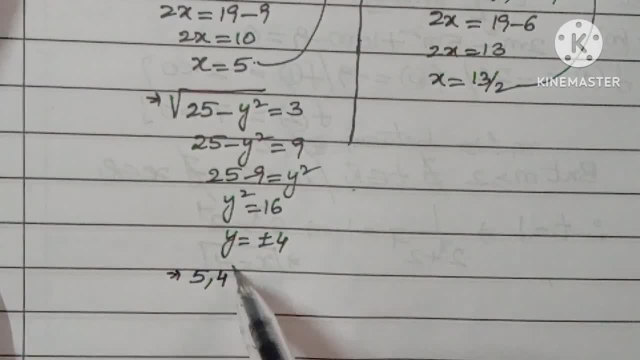 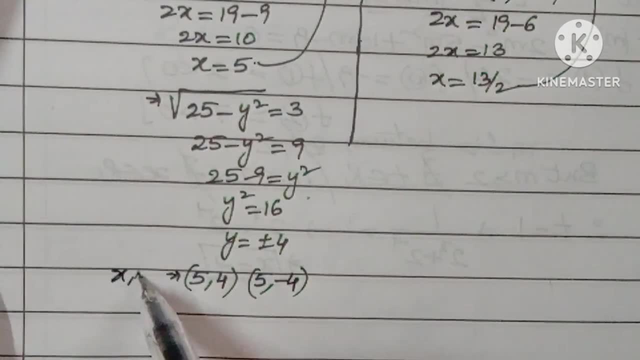 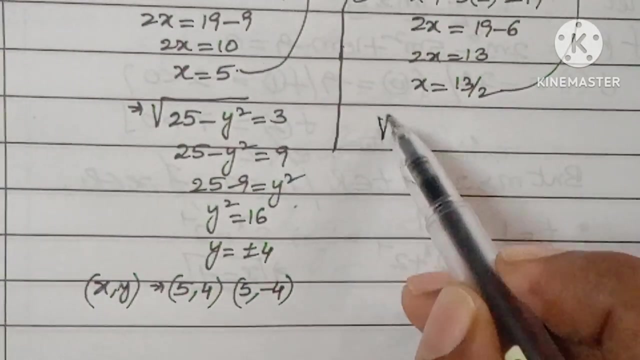 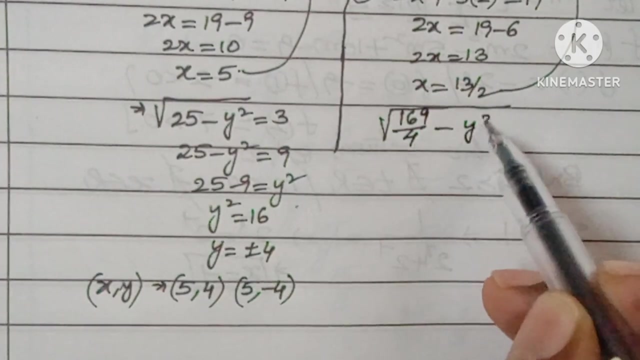 now you are getting the answer. you are getting the values of x, y, 5 comma, 4, 5 comma minus 4, x comma, y values. you are getting two values here. now, if you take the second one, square root of 169 by 4 minus y square is equal to 2 squaring on both sides.